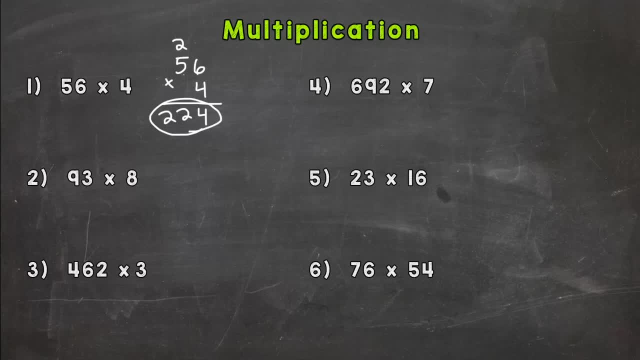 a multiplication problem. So number 2: we have 93 times 8.. So we start with 8 times 3.. 8 times 3 is 24,. carry the 2.. Then we do 8 times 9, which is 72,. 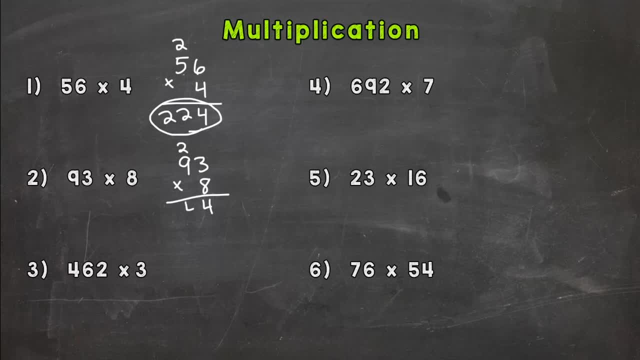 82,. plus that two is 74.. Circle our product: 744.. Now number three. we have a three digit number by a one digit, So a little bit different, but it's the same exact process. We just have an extra number here, So we need to take the three to the two, the six and the four. 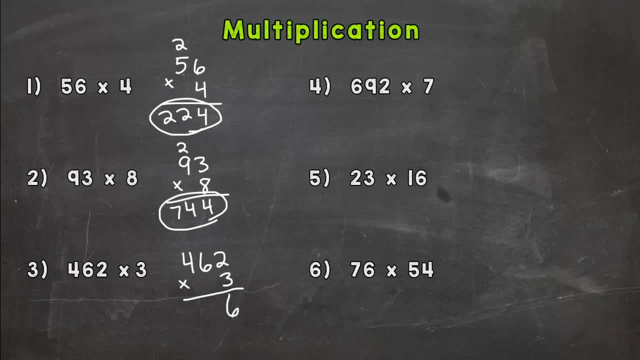 So we start with three times two, which is six, Then we do three times six, which is 18, carry the one. Next we do three times four, which is 12, plus that one is 13.. So our product is 1,386.. 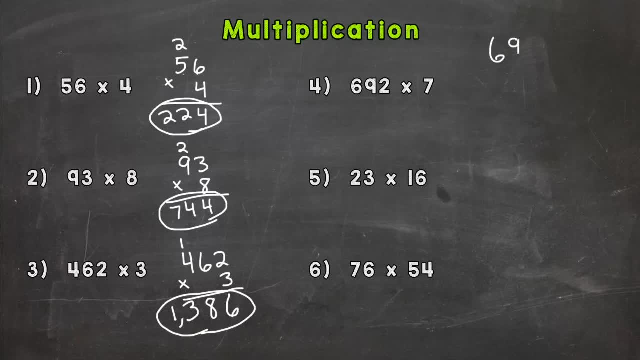 Number four: here we have 692.. 792 times seven. So we need to take the seven to the two, the nine and the six. So let's start with seven times two, which is 14.. Seven times nine is 63, plus that one is 64.. 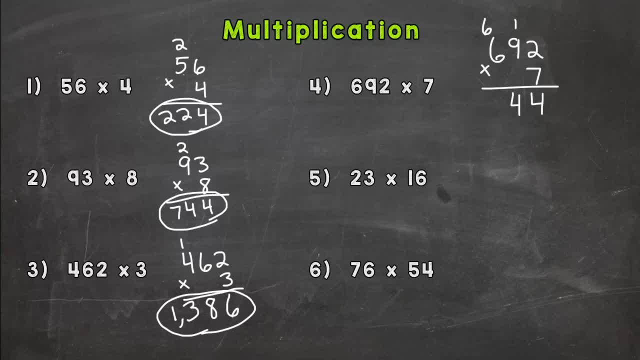 Now we have seven times six, which is 42,, plus that six is 44. So this is 23 all together. There's goes our other, foured by a one digit number, when we really had to substitute those three numbers. So four three gives us four thousand, so I set it up to 7, it has to be 24,. 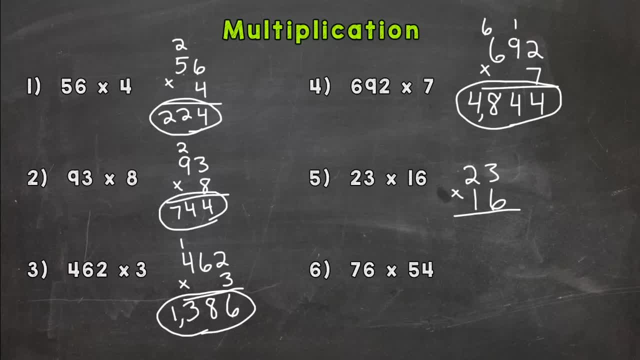 five is 38. So 4,844,. the next 3, we should have 8, by multiplying the 6 times 3 and then 6 times 2.. So it's the same exact stuff we've been doing. So 6 times 3 is 18.. 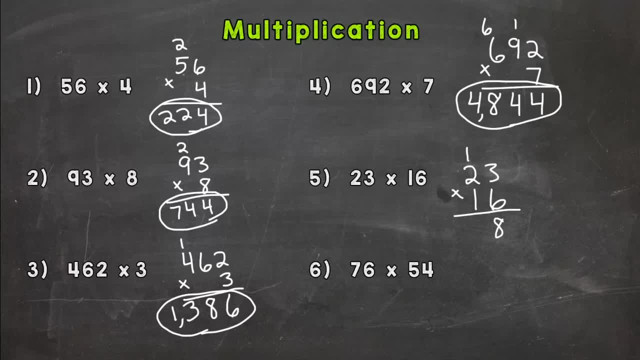 Carry the 1.. 6 times 2 is 12, plus that 1 is 13.. This is not our answer. We're not quite done yet. That's part of our answer, but not quite done. We're done with the 6, though, so I like crossing it off. 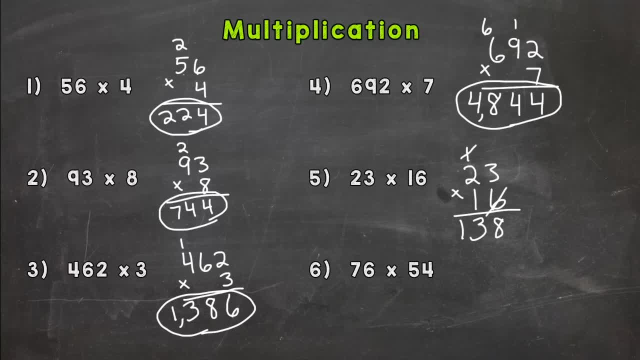 It shows we're done, and we are also done with this 1 that we carried. So I like to cross that off so we don't get confused later if we have other numbers up there. Now the next step is very, very important. 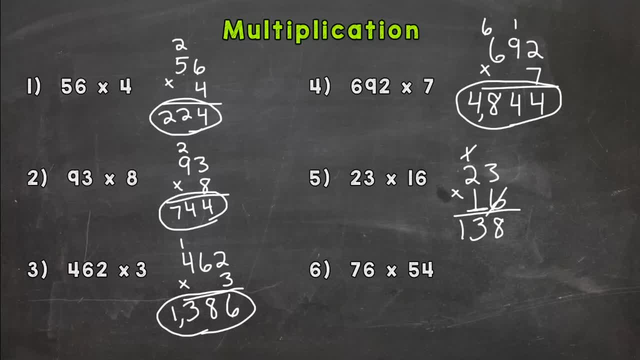 This 1 right here that I'm underlining, that is in the 10s place. It is worth 10.. So we need a 0 here to make it. so we are multiplying that 12.. 23 up top by 10.. 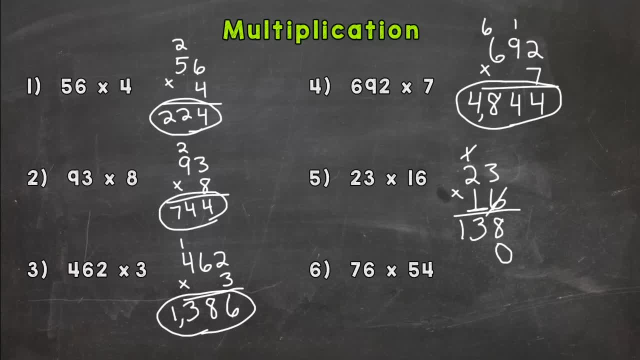 It's pushing everything to the right place value when we take the 1 to the 3 and then the 2.. So we start here by doing 1 times 3, which is 3.. Then we take the 1 to the 2.. 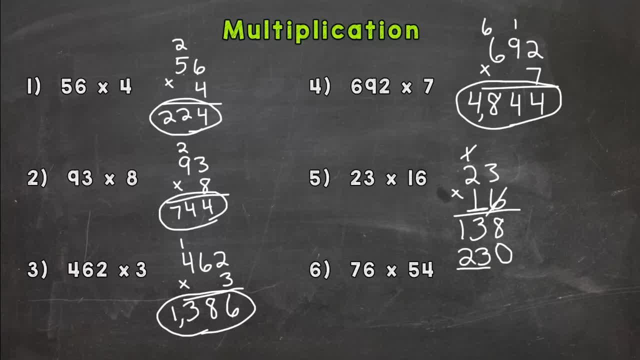 1 times 2 is 2.. And then we add these two numbers: 8 plus 0 is 8.. 3 plus 3.. 3 is 6. And then 1 plus 2 is 3.. So our answer is 368, our product. 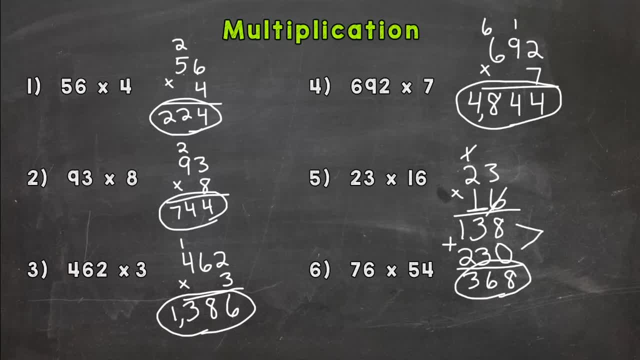 Now these two numbers that we added together. these are called partial products And we add them together to get our product. So let's do number 6, another 2 by 2.. And I'm going to come over here to the side where I have more room. 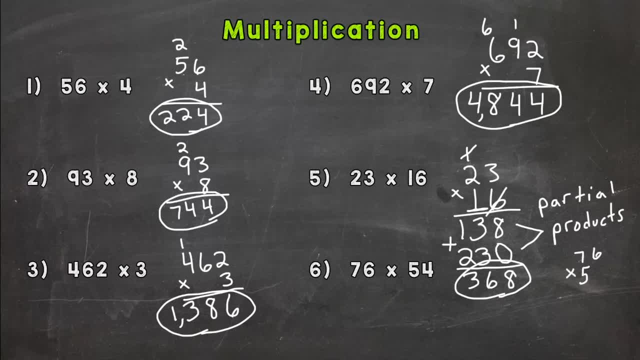 So I have 76 times 54. So I need to start by taking my 4 to the 6 and 4 to the 7.. 4 times 6 is 24.. Carry the 2. 4 times 7 is 28 plus 2 is 30..